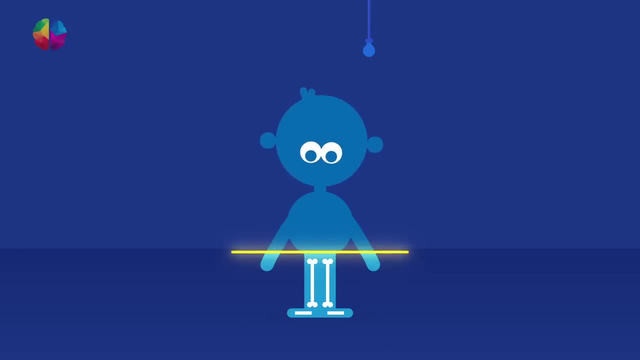 above your knees. They might feel tired if you've been doing a lot of running. If they do, that is fine. Don't be annoyed by this. It is not a bad thing. Just recognise how they feel and accept it. Now the scanner is on your tummy. Is there any rumbling there? 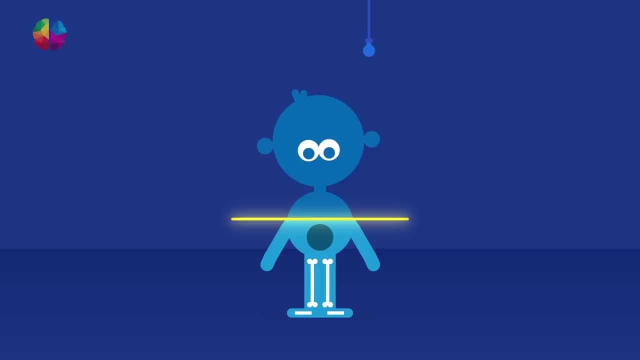 Can you feel your food being digested? Be open to any other feelings or sensations there. Now the scanner has moved up to your chest and around your heart. Focus on this area. Think about what you can feel there, Now onto your shoulders and neck. Is there any tingling there, Any tightness? Remember. 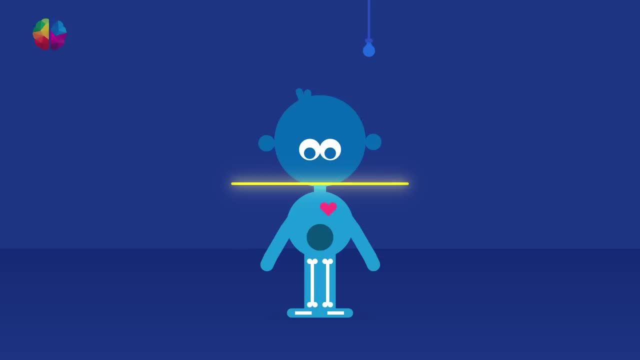 that any feelings are okay. We are just recognising what is going on. The scanner is moving over your face now Think about your chin, Your lips. Are these relaxed or shaky? Shut tight Your cheeks, Your eyes, Your forehead.